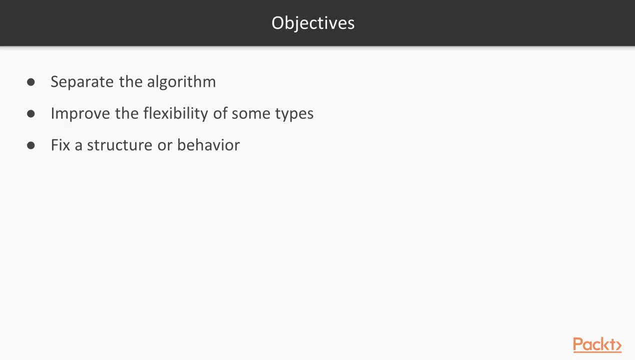 stored in the object. With Behavioral Design Patterns, we are mainly dealing with algorithms. Visitor Patterns are not an exception. The objectives that we are trying to achieve are listed here. The first and foremost is to separate the algorithm of some type from its implementation. 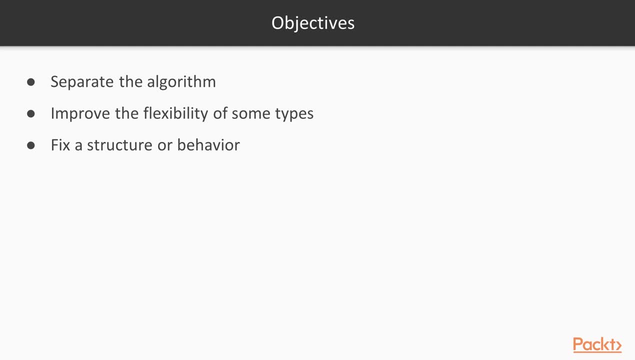 Secondly, to improve the flexibility of some types by using them with little or no logic at all, so all new functionality can be added without altering the object structure. And lastly, to fix a structure or behavior that would break the open or closed principle in a type. 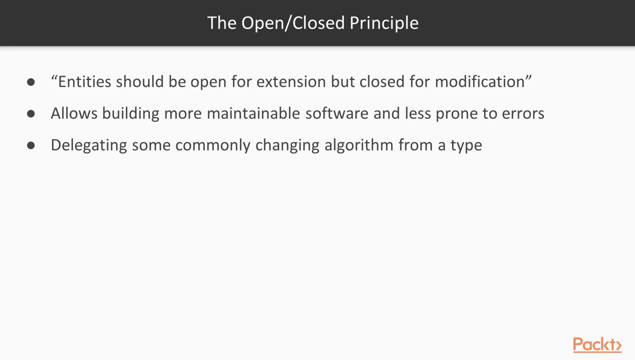 You might be thinking what the open or closed principle is In computer science. the open or closed principle states that entities should be open for extension but closed for modification. This simple statement has lots of implications that allows building more maintainable software and less prone to errors. 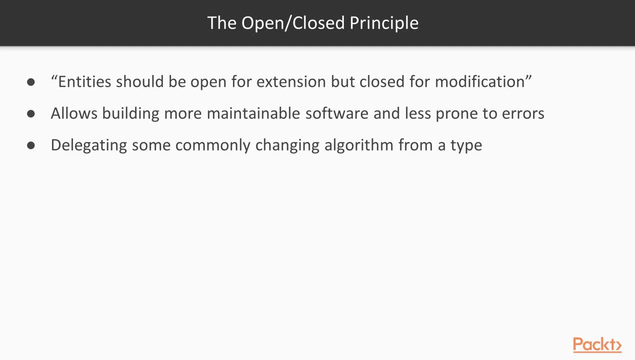 And the Visitor Pattern helps us to delegate some commonly changing algorithm from a type that we need to be stable to an external type that can change, often without affecting our original one. We are going to develop a simple log appender as an example of the Visitor Pattern. 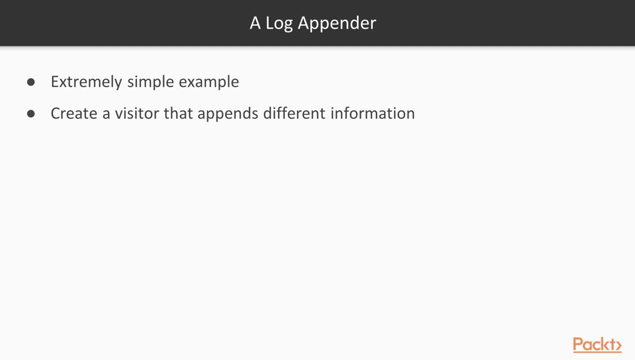 Following the approach, we have had a lot of problems with the Visitor Pattern, As we have said in previous sections. we will start with an extremely simple example to clearly understand how the Visitor Design Pattern works, before jumping to a more complex one. We have already developed similar examples, modifying texts too, but in slightly different. 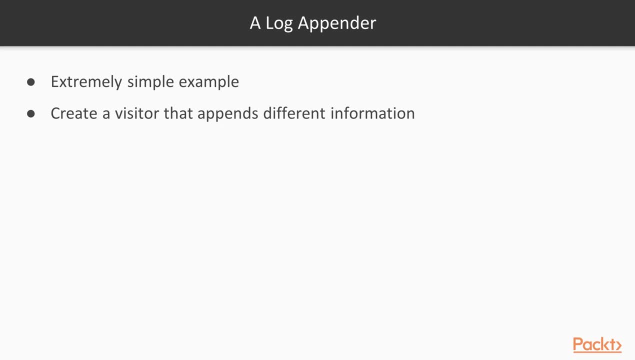 ways. For this particular example, we will create a visitor that appends different information to the types it visits. To effectively use the Visitor Design Pattern, we must have two roles: a visitor and a visitable. The visitor is the type that will act within a visitable type, So a visitable interface. 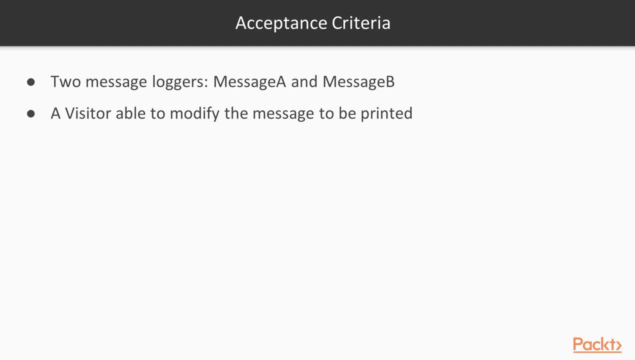 implementation has an algorithm detached to the visitor type, So we need two message loggers, message A and message B, that will print a message with an A or B respectively before the message. Also, we need a visitor to be able to modify the message to be printed. 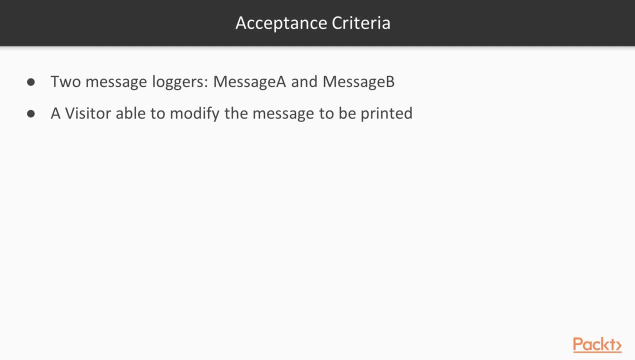 It will append the text visited A or visited B to them respectively. Now that you are well aware of what we want to do in this video, let's start with the unit tests. As we mentioned before, we will need a role for the visitor and the visitable interfaces. 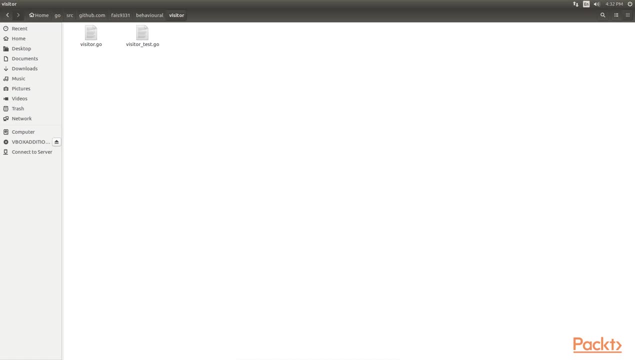 They will be interfaces. We also need the message A and message B structs. I have created two files- visitorgo and visitor underscore- testgo- within the folder named visitor. Open the file visitorgo. Let's start adding the code. First we add the package. 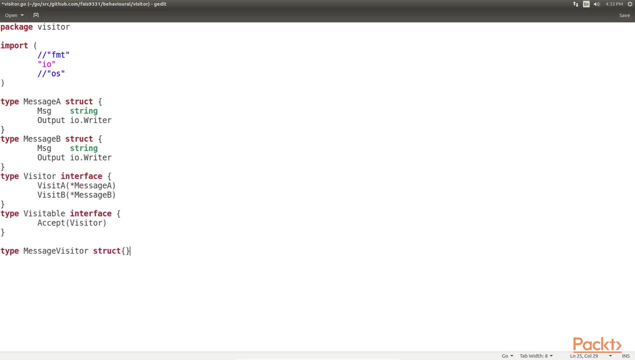 name: import statement structs and interfaces. The types message A and message B structs both have a message field to store the text that they will print. The output iowriter will implement the osstdout interface by default or a new iowriter interface like the one. 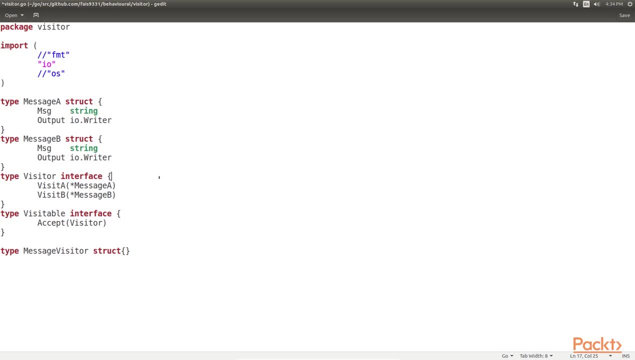 we will use to check the contents are correct. The visitor interface has a visit method, one for each of visitable interfaces: message A and message B type. The visitable interface has a method called acceptVisitor that will execute the decoupled algorithm. Like in previous examples, we will create a type that implements the iowriter. 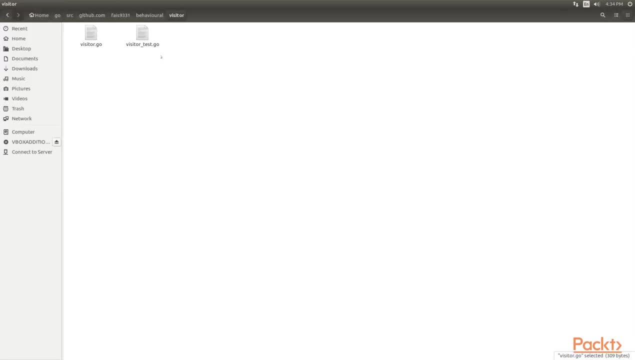 package so that we can use it in tests, Close this file and move to the visitorTestgo file. Here we first add the package name testingHelper struct and a function testHelper. The testHelper struct implements the iowriter interface. Its functionality is quite simple. 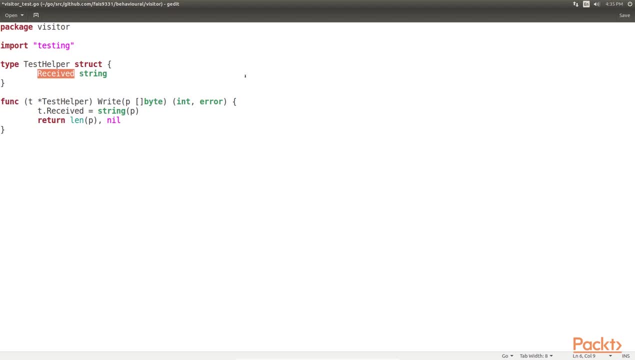 it stores the written bytes on the received field. Later we can check the contents of received to test against our expected value. We will write just one test that will check the overall correctness of the code. Within this test we will write two subtests, one for message A and one for message B. types: 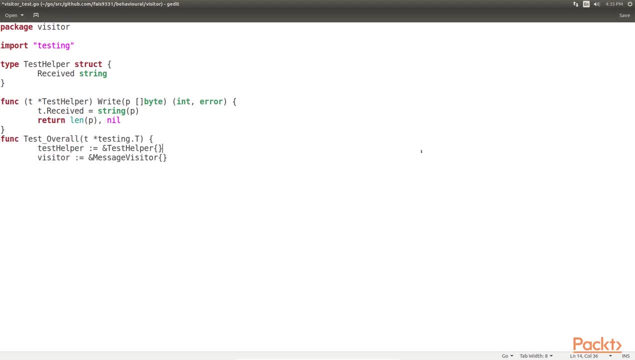 Let's do this. Ok, we will use a testHelper struct and a messageVisitor struct on each test for each message type. Now let's first add the code to test the message. The messageA type Done. This is the full first test. We created messageA struct giving 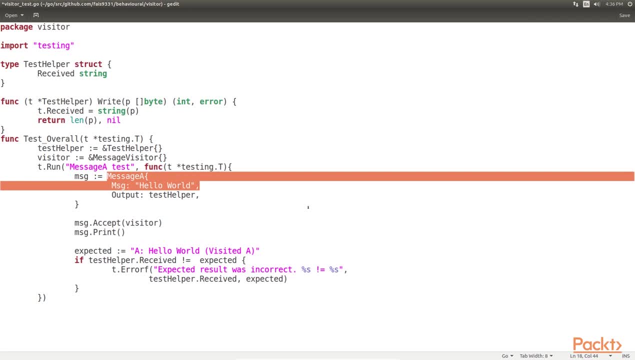 it a value helloWorld for the message field and the pointer to testHelper which we created at the beginning of the test. Then we execute its accept method Inside the acceptVisitor method. on the messageA struct, the visitA message is executed to alter the contents. 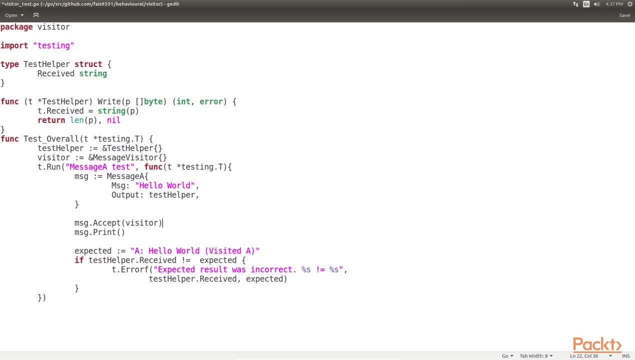 of the message field. That's why we passed the pointer to visitA method. Without a pointer, the contents won't be persisted To test. if the visitA type has done its job within the accept method, we must call the print method on the messageA type later. This way, the messageA struct must write the contents. 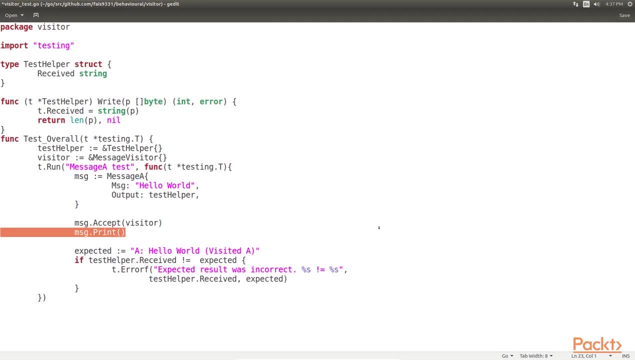 of msg to the provided IOwriter interface. that is, our testHelper. The last part of the test is the check. According to the description of the acceptance criteria. two, the output text of messageA type must be prefixed with the text A, The stored message and the text visited just at the end. So for the messageA type, the 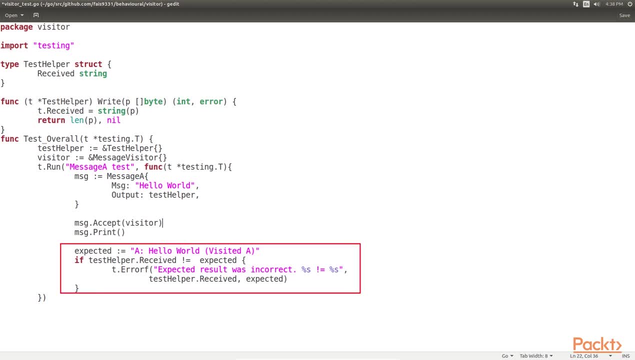 expected text must be in double quotes. A colon helloWorld- and in parenthesis- visited. This is the check that we did in the if section. The messageB type has a very similar implementation. Let's write the code for messageB type: 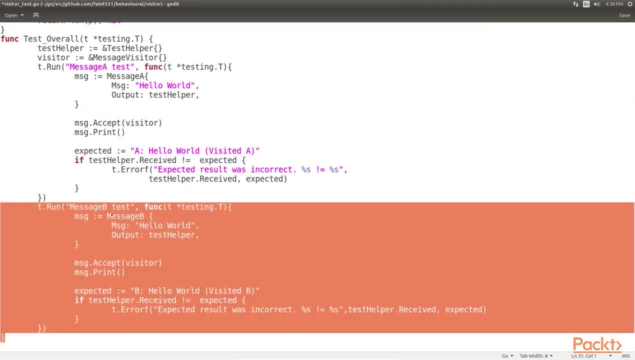 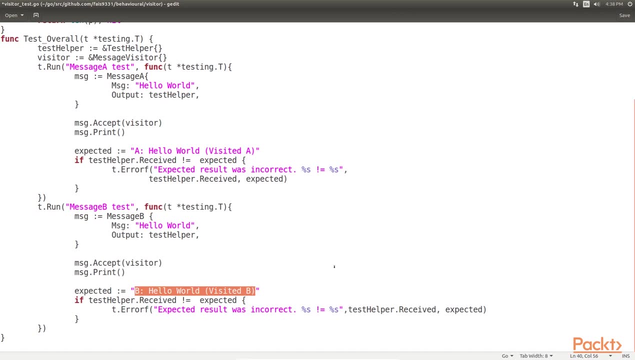 In fact, we have just changed the type from messageA to messageB and the expected text now is bhelloWorld. The message field is also helloWorld and we also used the testHelper type. We still lack the correct implementations of the interfaces to compile the code and run. 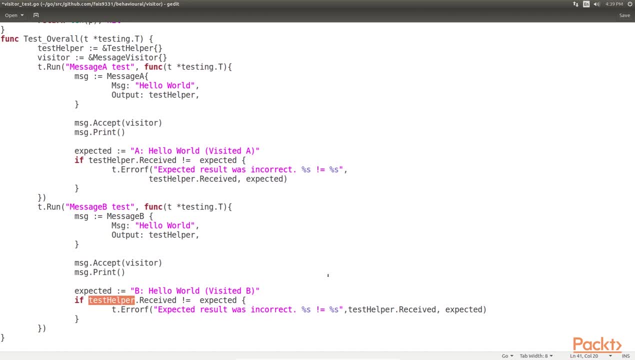 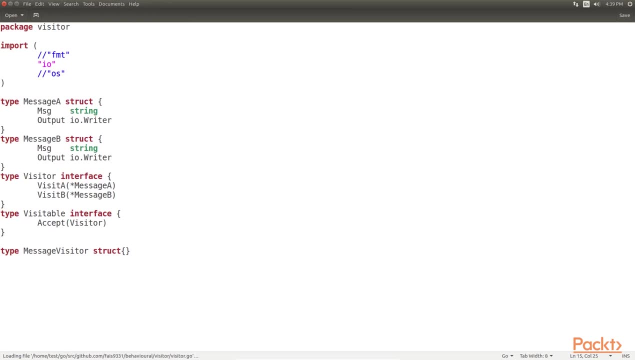 the tests. The messageA and messageB structs have to implement the acceptVisitor method. Let's save this file and go back to our visitorgo file. So here let's add the code to implement the acceptVisitor method for messageA and messageB. 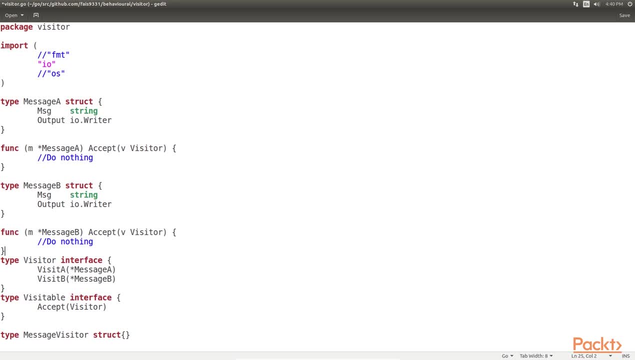 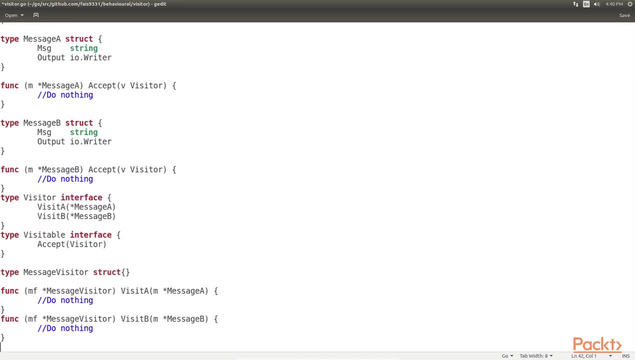 We then add the code for the implementations of the visitA method for messageA and messageB that are declared on the visitor interface. The message visitor interface is the type that must implement them. Finally, we will create a print method for each message type. 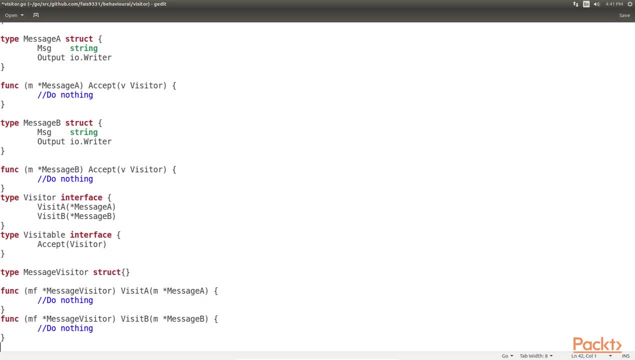 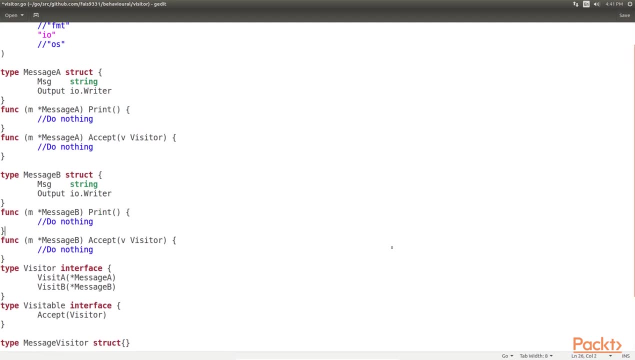 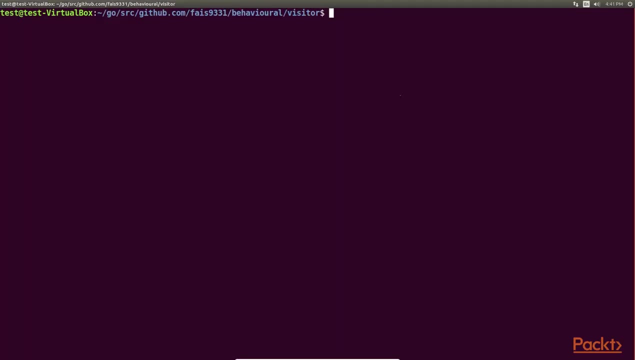 This is the method that we will use to test the contents of the message field on each type. Let's do it Now. we can run the tests to really check if they are failing. Thanks for watching yet So let's save the file. Open the terminal. Run the command gotest-v. The outputs of the 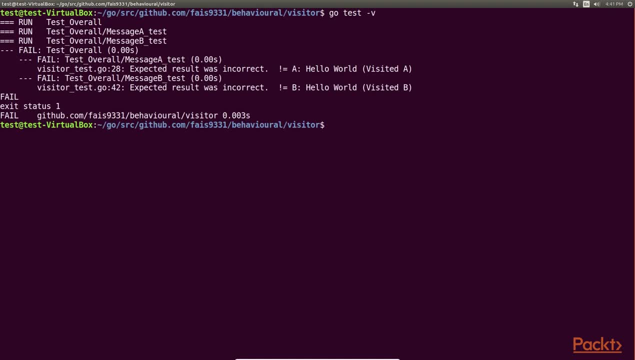 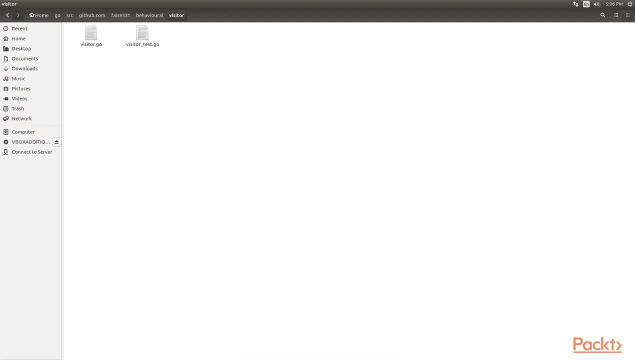 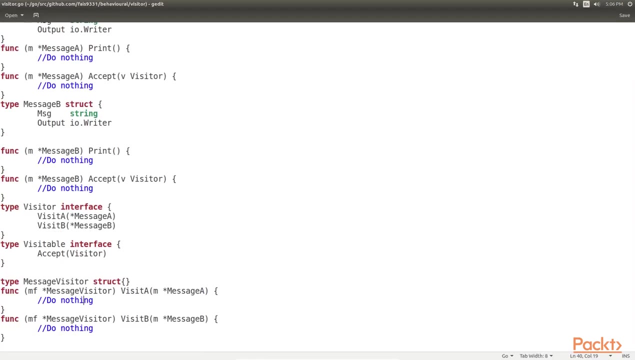 tests are clear. The expected messages were incorrect because the contents were empty. It's time to create the implementations. We will start completing the implementation of the visitA message A and visitB message B methods. Open the visitorgo file In the type message visitor struct, add this line: Similarly, we do this for messageB Cool. 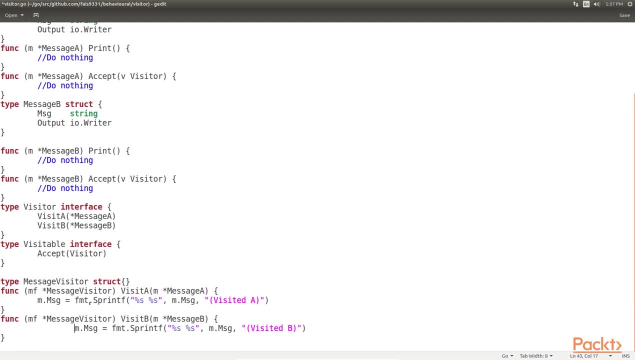 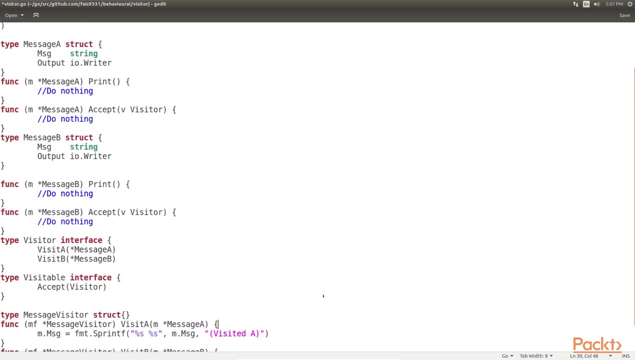 Its functionality is quite straightforward. The fmtsprintf method returns a formatted string with the actual contents of mmessage, a white space and the message visited. This string will be stored on the message field, overriding the previous contents. Now let's 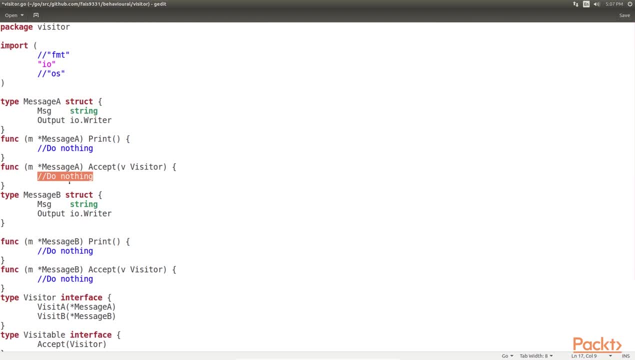 develop the accept method for each message type that must execute the corresponding message. This small code has some implications on it. In both cases we are using a visitor which, in our example, is exactly the same as the message-visitor interface. but they could. 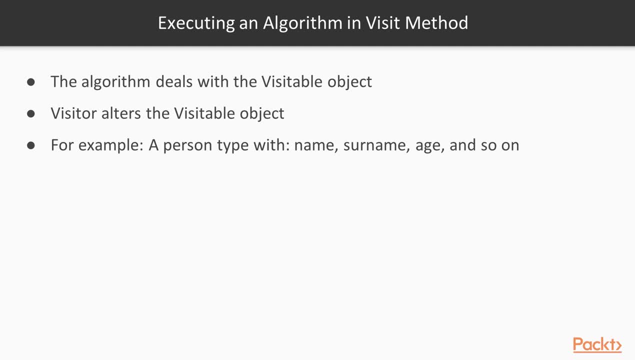 be completely different. The key is to understand that the visitor pattern executes an algorithm in its visit method that deals with the visitable object. What could the visitor be doing In this example? it alters the visitable object, but it could be simply fetching information. 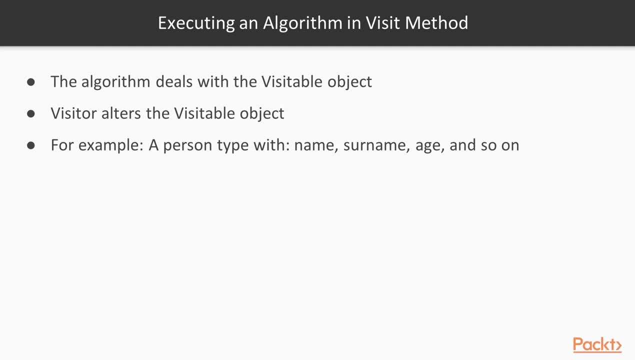 from it. For example, we could have a person who is a visitor. We could have a person who is a person type with lots of fields: name, surname, age, address, city, postal code and so on. We could write a visitor to fetch the name and the surname from a person as a unique. 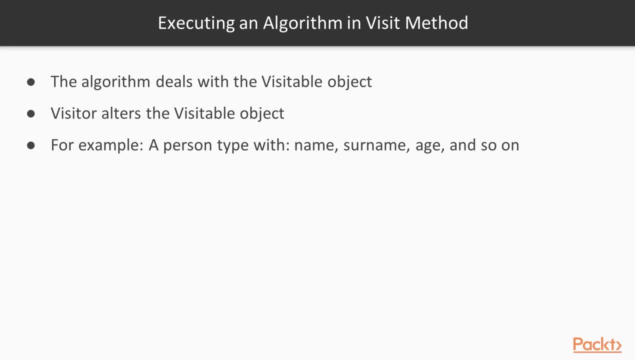 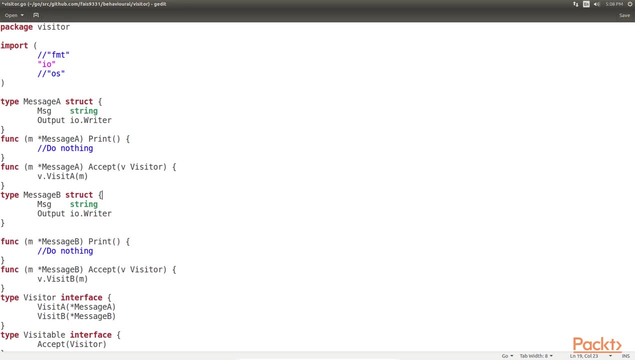 string a visitor to fetch the address info for different sections of an app, and so on. Finally, there is the print method, which will help us to test the types We mentioned before that it must print to the std out call by default. Let's add the print method next. 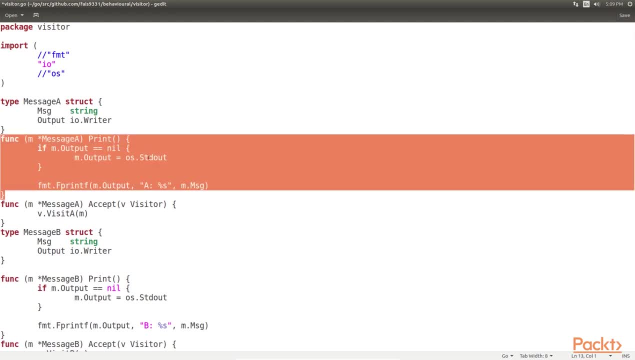 It first checks the contents of the output field to assign the output of the osstd out call. in case it is null In our tests, we are storing a pointer there to our test helper type. so this line is never executed in our test. Finally, each message type prints to: 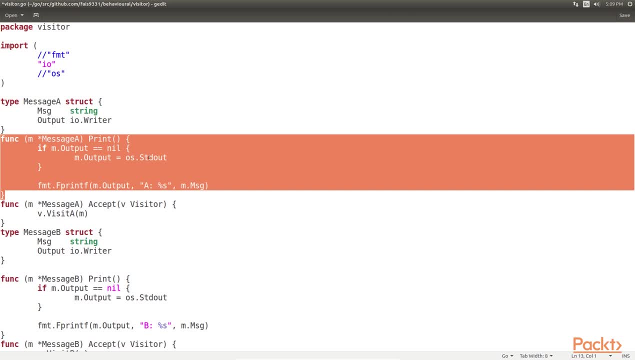 the output field the full message stored in the message field. This is done by using the fprintf method, which takes an iowriter package as the first argument and the text to format as the next argument. Before you save the file, remember to include fmt and. 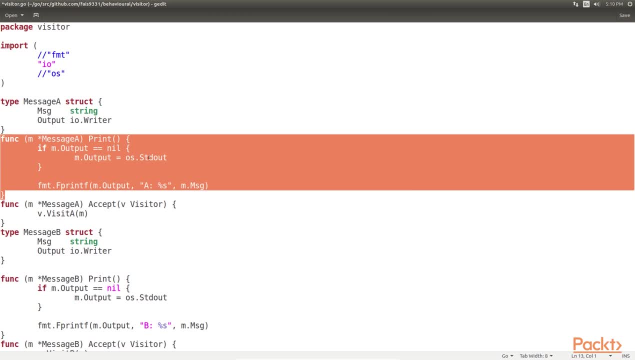 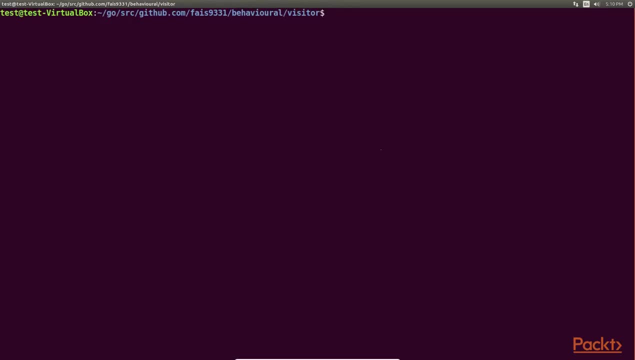 os in the import statement. Our implementation is now complete and we can run the tests again to see if they all pass. Now save the file, Move to the terminal and run the command gotest-v. Everything is okay. The visitor pattern has done its job flawlessly and the 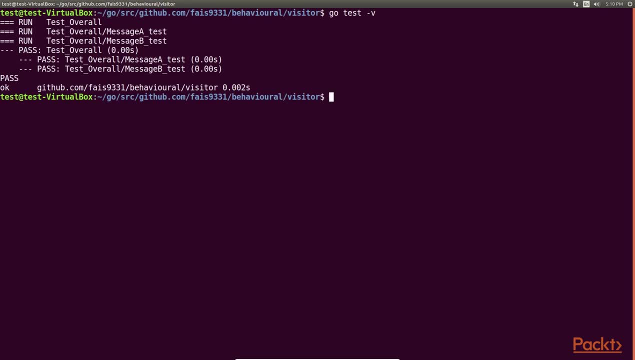 message contents were altered after calling their visit methods. The visitor pattern is now okay. important thing here is that we can add more functionality to both the structs message A and message B, without altering their types. We can just create a new visitor type that does everything on the visitable. For example, we can create a 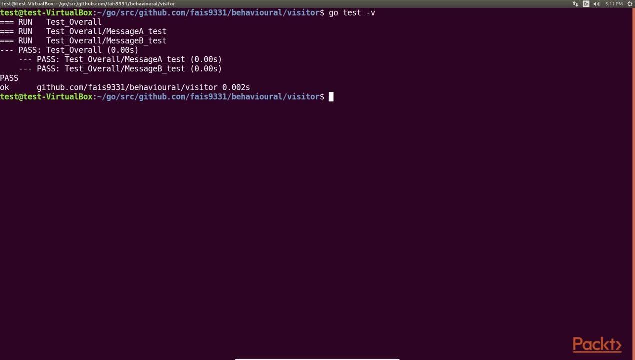 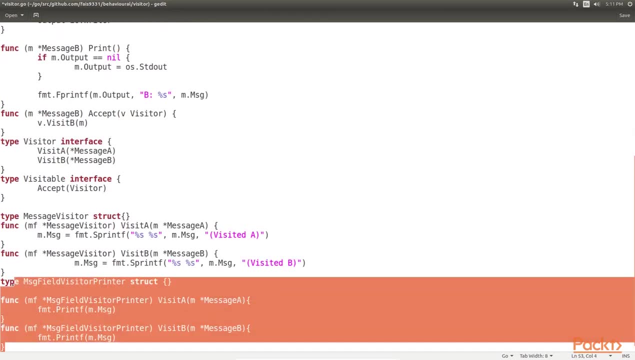 visitor to add a method that prints the contents of the message field. Let's go back to visitorgo. At the end of the code add the message field: visitor printer struct. So we have just added some functionality to both types without altering their contents. That's the power of the visitor design pattern Now. 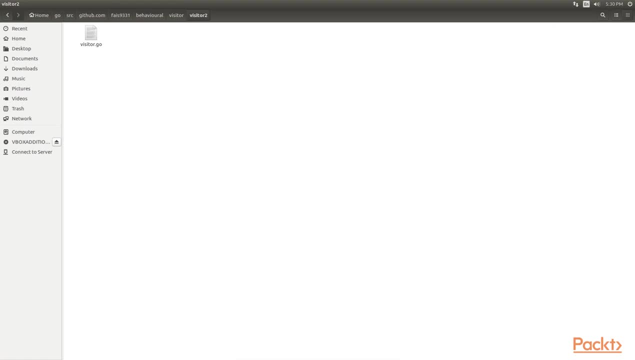 we will develop a second example, this one a bit more complex. In this case, we will emulate an online shop with a few products. The products will have plain types with just fields, and we will make a couple of visitors to deal with them in the group. First of all, we will develop the interfaces: Open visitorgo. 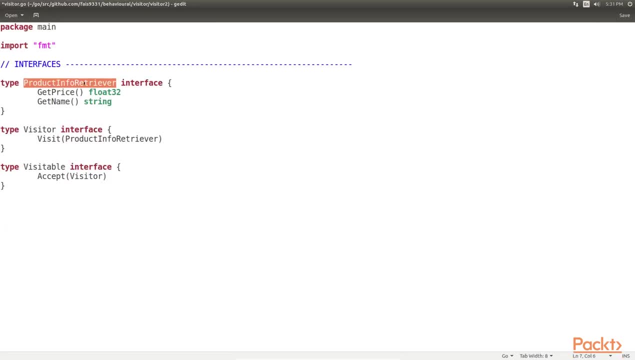 and the interfaces. The product info retriever type has a method to get the price and the price equals the price. This is a new type that we will use to and the name of the product. The visitor interface, like before, has a visit method that accepts the product info. 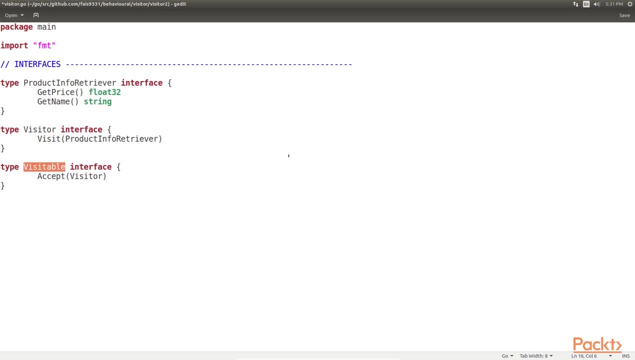 retriever type. Finally, visitable interface is exactly the same. It has an accept method that takes a visitor type as an argument. All the products on the online shop must implement the product info retriever type. Also, most products will have some common fields, such as name or price. 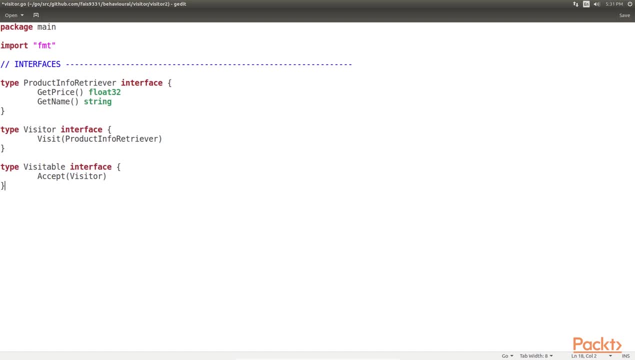 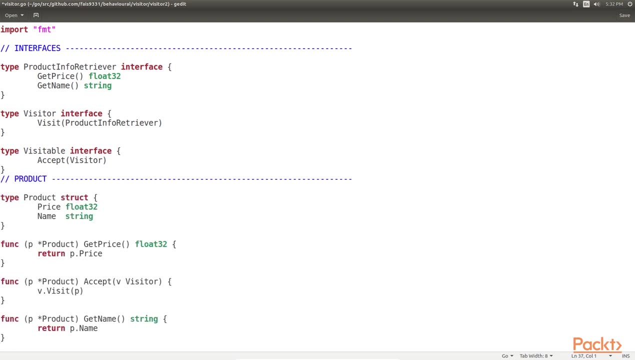 Now we'll create the product type, Select the product info, receiver and visitable interfaces and embed it on each product. Let's do it Now. we have a very generic product type that can store the information about almost any product of the shop. For example, we could have a rice and pasta product. 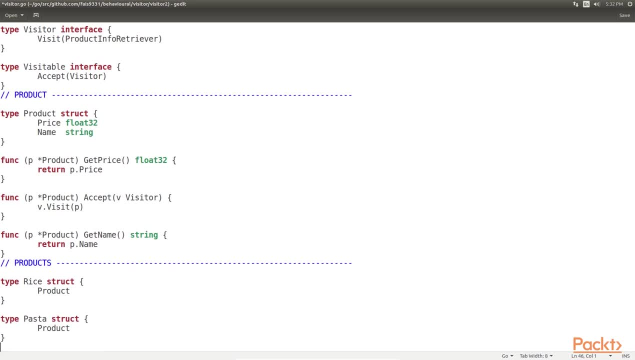 So next we add the rice and pasta struct. Each has the product type embedded. Now we need to create a couple of visitors interfaces: one that sums the price of all products and one that prints the name of each. Here we add the code for it. 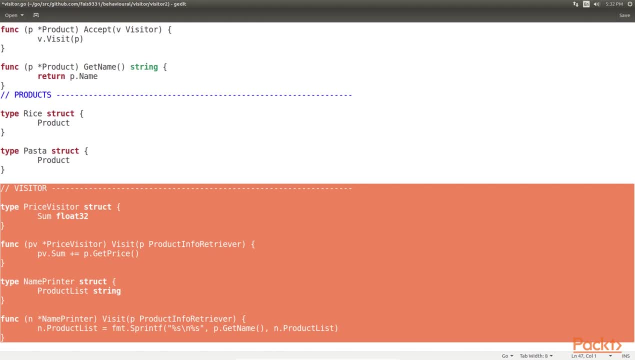 The price visitor struct takes the value of the price variable of the product info retriever type passed as an argument and it adds it to the sum field. The name printer struct stores the name of the product info retriever type passed as an argument and appends it to a new line on the product list field. 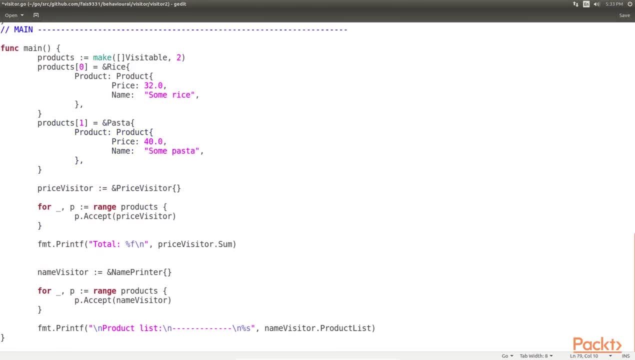 Time for the main function. Let's add the main function. We create a slice of two visitable objects, A rice and pasta type, A rice and pasta type with some arbitrary names. Then we iterate for each of them using a price visitor instance as an argument. 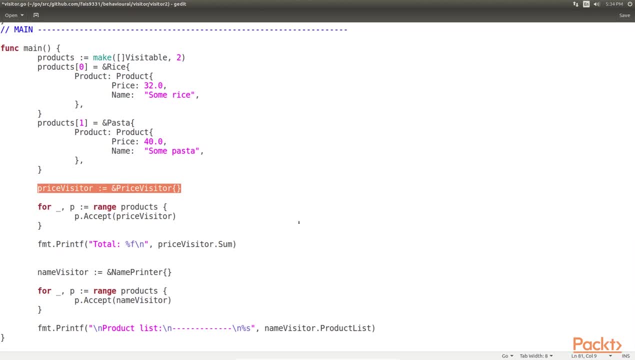 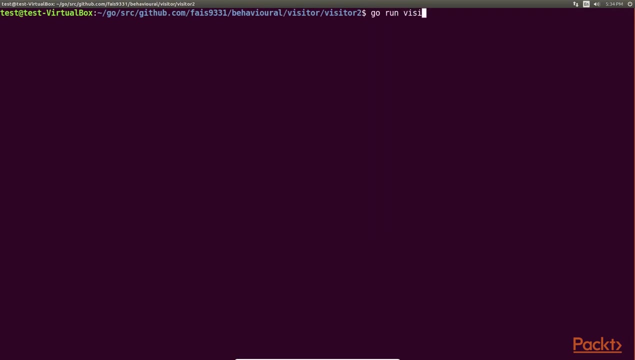 We print the total price after the range 4.. Finally, we repeat this operation with the name printer and print the resulting product list. Let's go ahead and check the output of this main function, Save the file and move to the terminal Type the command gorunvisitorgo. Ok, this is a nice example of the visitor pattern. 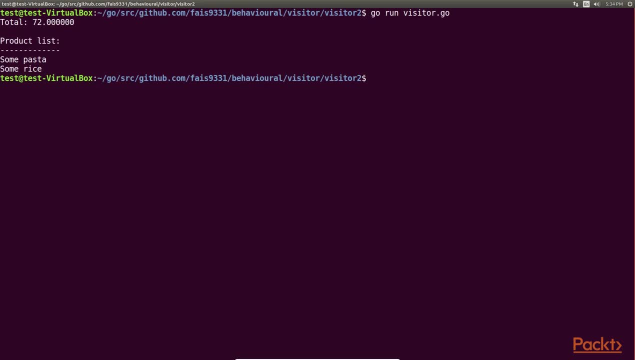 but what if there are special considerations about a product? For example, what if we need to sum 20 to the total price of a fridge type? Ok, let's write the fridge structure. Let's go back to visitorgo and write the fridge structure. 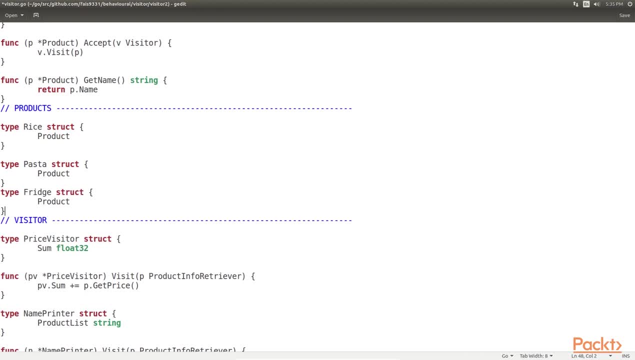 Over here. The idea here is just to override the getPrice method to return the product's price plus 20.. For this we add the next lines of code. Unfortunately, this isn't enough for our example. The first line of code is not enough for our example. 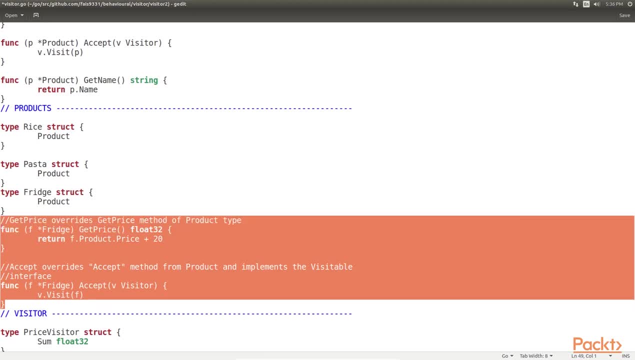 The first line of code is not enough. for our example, The fridge structure is not of a visitable type, The product struct is of a visitable type and the fridge struct has a product struct embedded, but, as we mentioned in earlier sections, a type that embeds a second type cannot be. 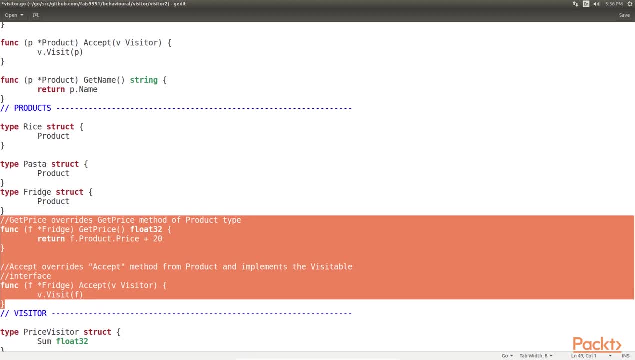 considered of that latter type, even when it has all its fields and methods. The solution is to implement the acceptVisitor method so that it can be considered as a visitable. Let's rewrite the main function: to add this new fridge product to the slice. 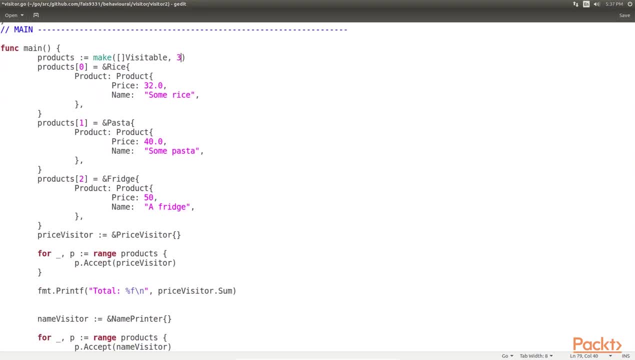 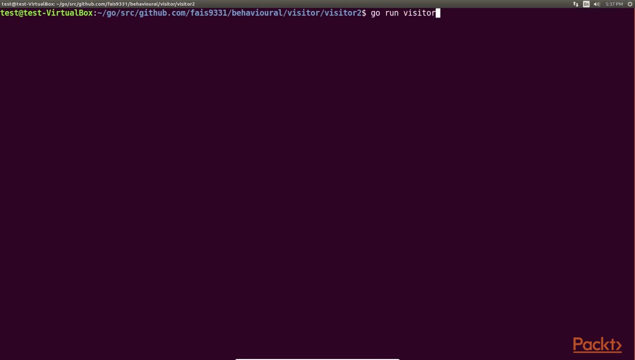 Since we added a third product, let's change this value to 3.. Everything else continues the same. running this new main function produces a different output. Let's run the test and check it First. save the file and move to the terminal. Run the command: gorunvisitorgo. 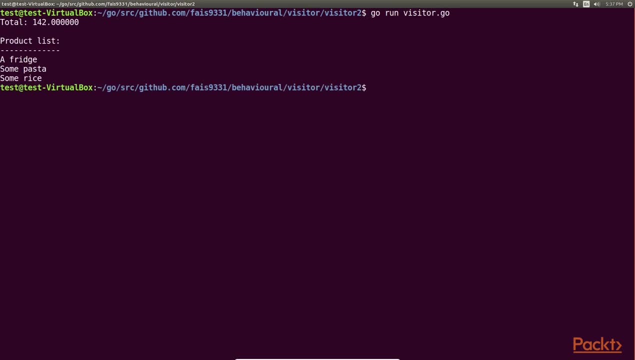 As expected, the total price is higher now, outputting the sum of the rice, the pasta and the fridge. We could be adding visitors forever to these products, but the idea is clear. We just need to run the test and check it. Let's see how this see the result. 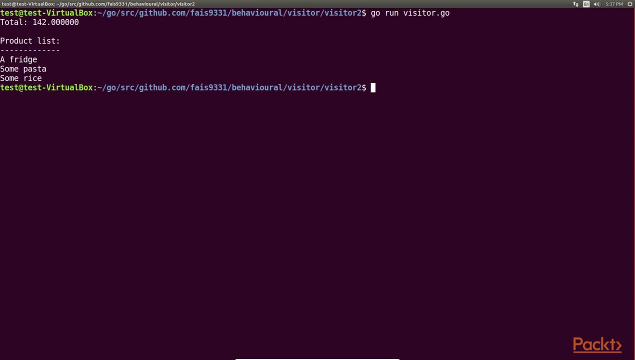 we decoupled some algorithms outside of the types to the visitors Superb. In this video we have seen a powerful abstraction to add new algorithms to some types using the visitor design patterns. 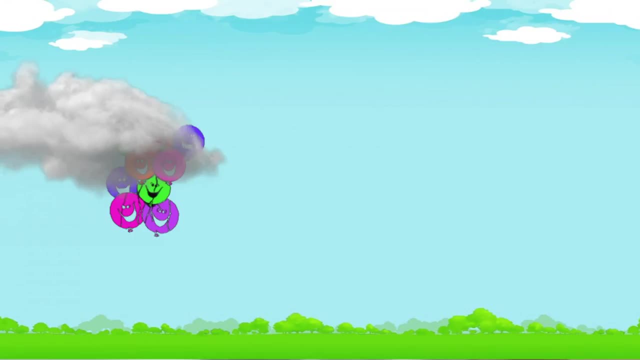 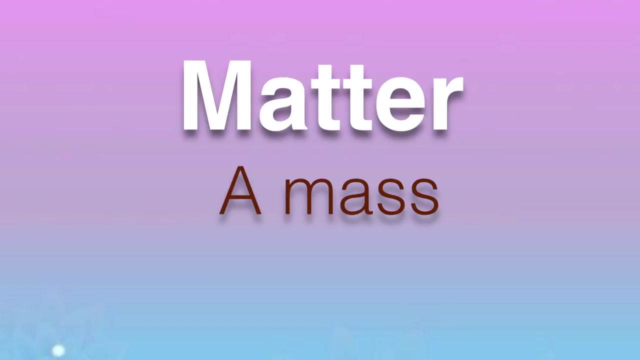 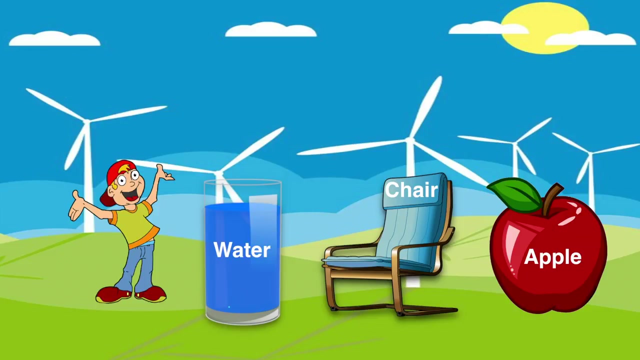 Whatever that you see around yourself is matter. Even the air that you don't see is matter. But what is this matter? A matter is anything that has a mass, a weight. Everything around you- water, chair, apple- has a weight, But they are so different from each other. 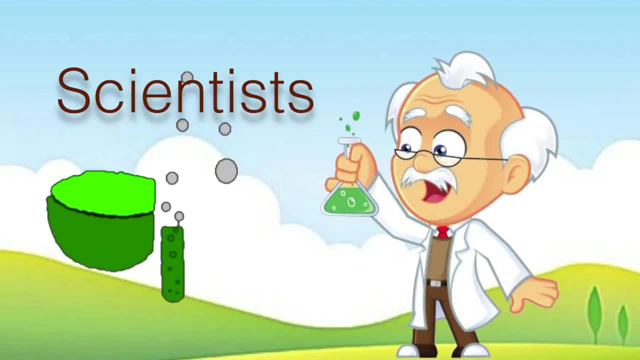 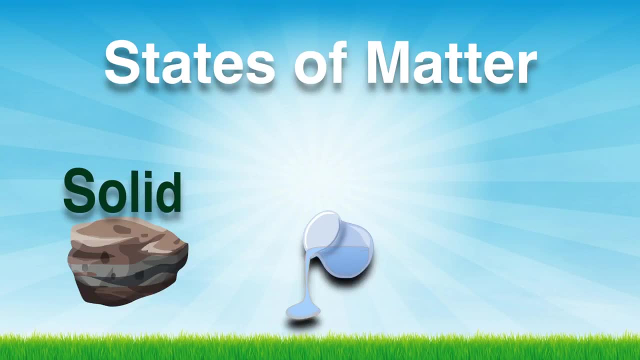 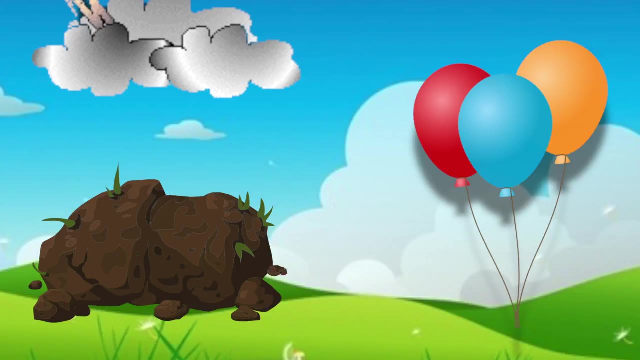 How do you categorize these things? Scientists thought about it before us and came to a decision that there are three states of matter: Solid, liquid and gaseous. You have heard these words before. What do they mean? Matter in solid state has a definite shape and size. It won't adjust. Take ice, for example. 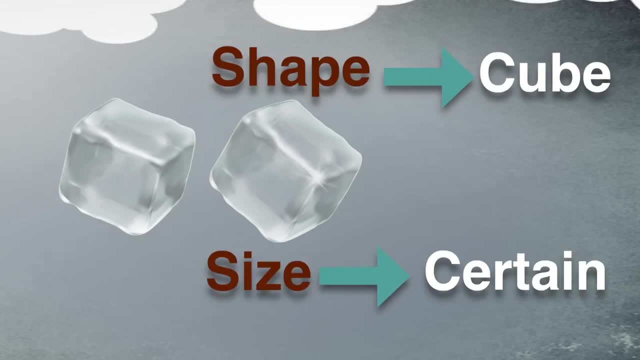 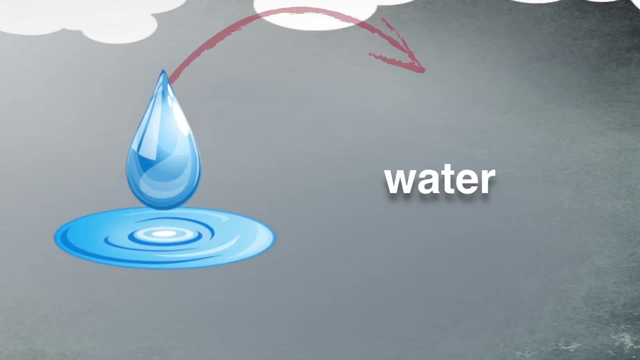 Definite shape is cube. size is also certain. Unless it melts, it won't adjust itself. When ice melts, it becomes water. Water adjusts Whichever beaker you put it in. it takes the shape of the beaker or the utensil. 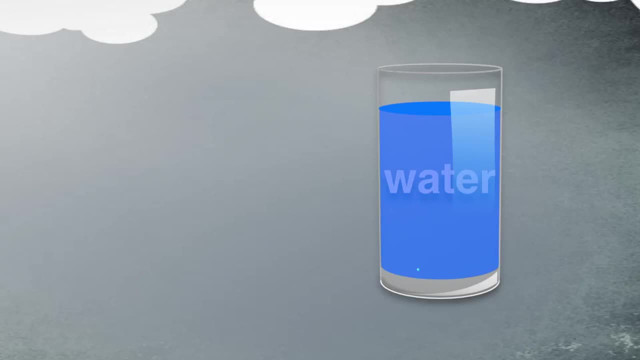 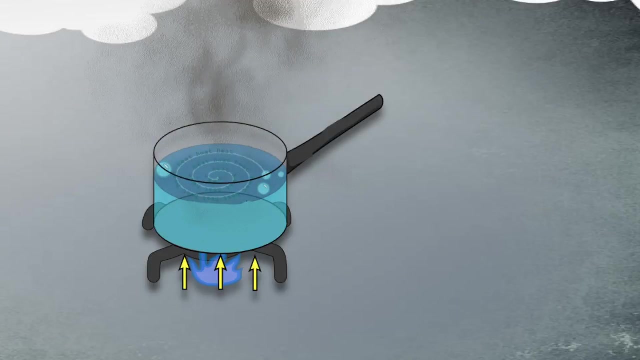 Water is the liquid state here. So no definite shape, but definite size. I mean 1 litre of water is still 1 litre, no matter where you put it in. Now, if you heat this water it becomes steam. Steam cannot be trapped. It is without a shape. 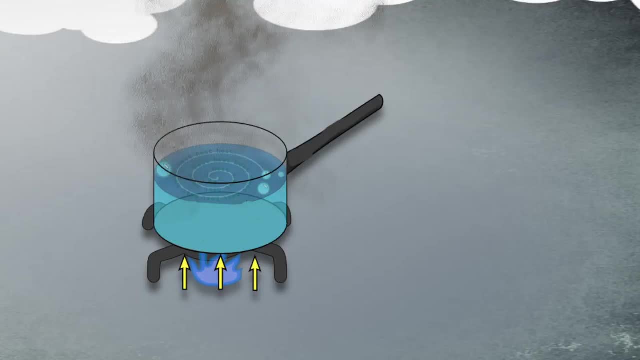 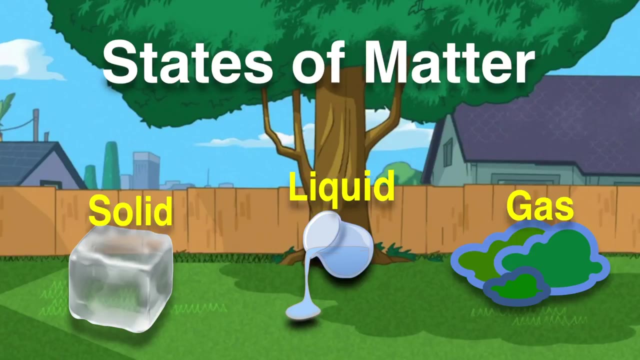 or a size. Whichever beaker you put it in, it will fill the whole place. Steam is truly the gas. Now you know the three states of matter. Which one is your favourite? Semi-stripe, sub-stripe, semitripe, sub-stripe and sub-stripe.